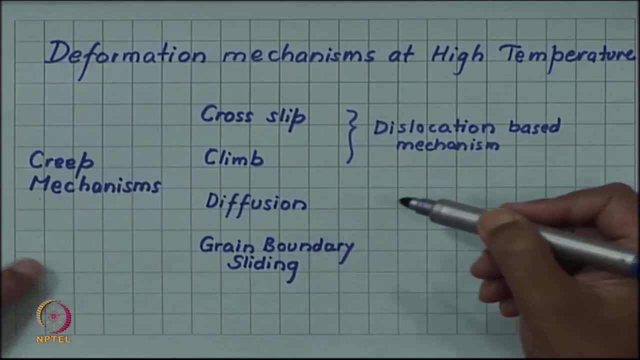 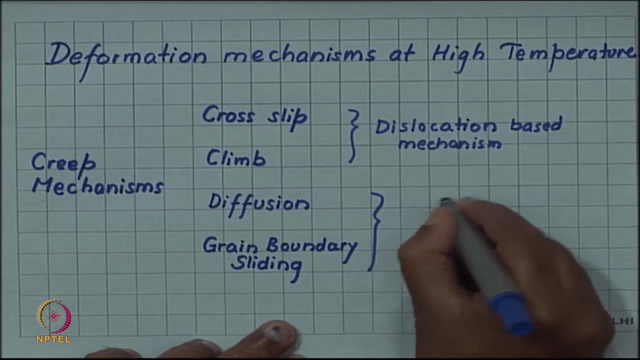 and grain boundary sliding. These are two mechanisms of plastic deformation which are not dislocation based, independent of dislocation, and they occur only at high temperature and do not happen at low temperature. So they are particularly effective in creep. So these are not based on dislocations. So 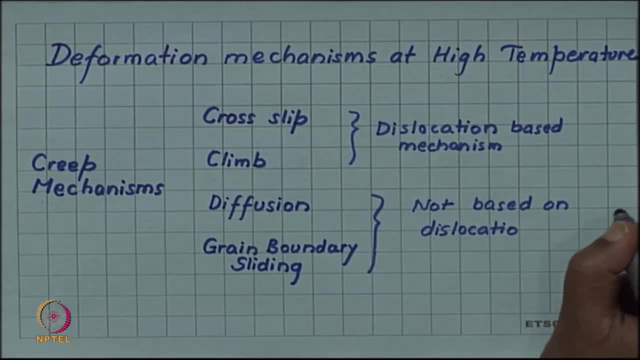 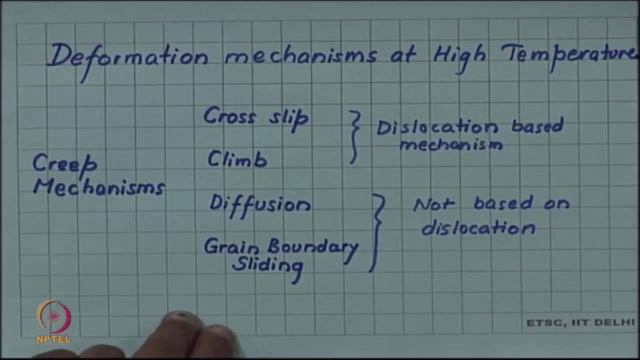 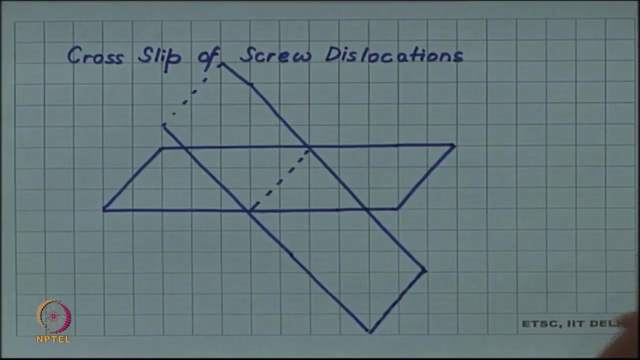 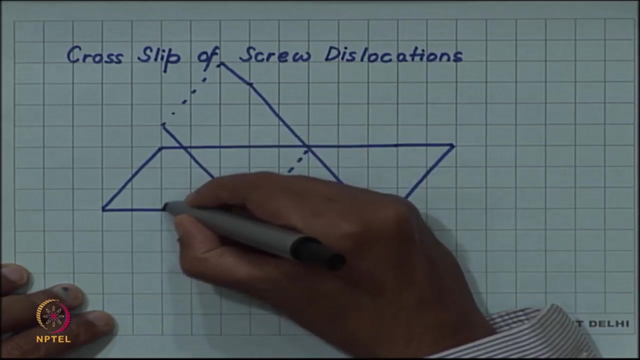 high temperature deformation. So this is the dislocation- need not necessarily be a dislocation based deformation. We have already seen a cross slip of a screw dislocations when we were discussing the dislocation- the topic of defects and dislocations- So let us say that this is a screw dislocation. we 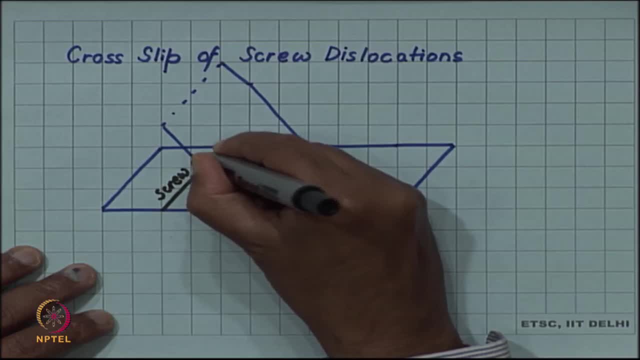 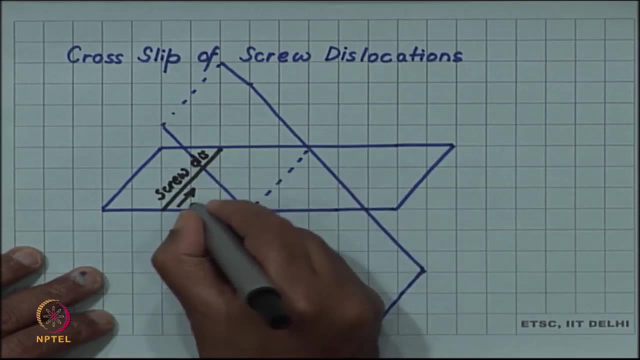 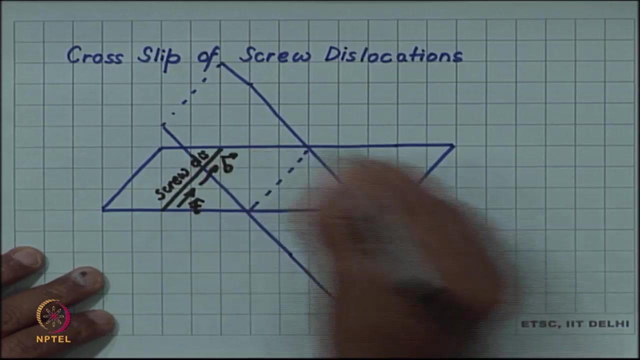 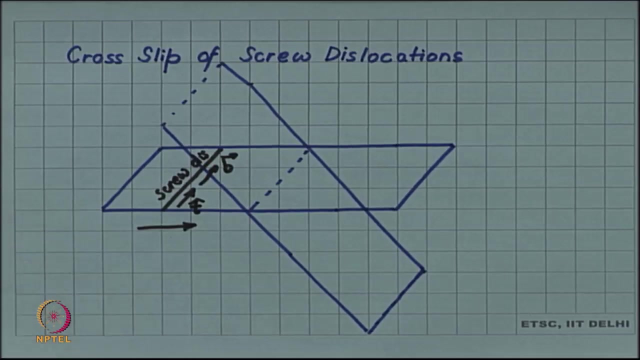 which was moving for. So if it is a screw dislocation, the T and B will be either parallel or anti parallel, So let me make parallel in this case. So if this dislocation was moving under the stress in this direction and suppose that the crystal contains some 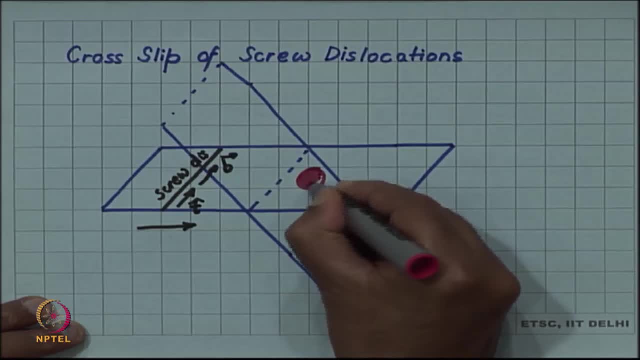 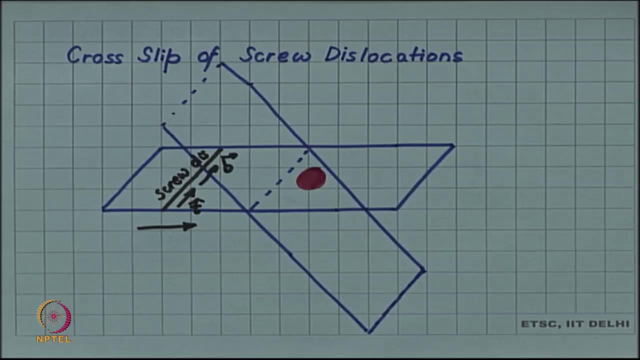 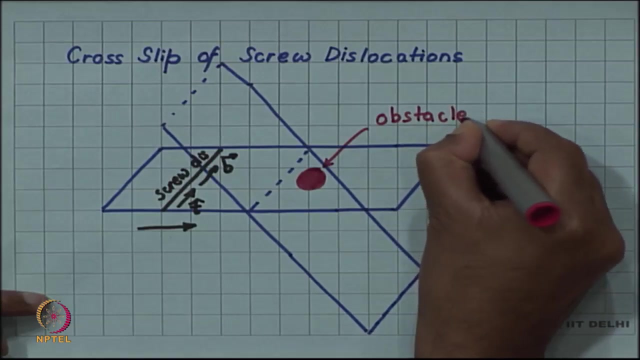 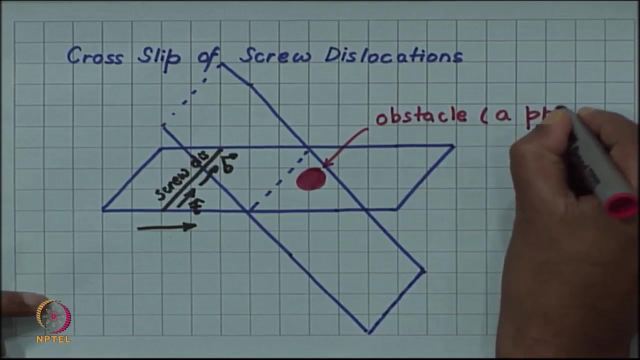 hard particles, reinforcement or precipitate. we have talked about precipitation, hardening. So suppose there is a precipitate sitting there and the dislocation cannot cut through. the precipitate cannot, So it acts as an obstacle. So this is an obstacle to dislocation motion. let us say a precipitate. So this dislocation? 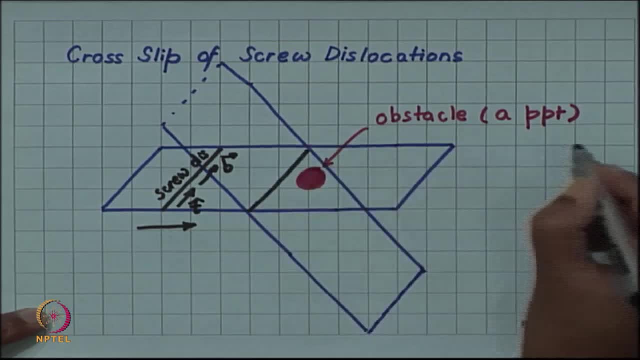 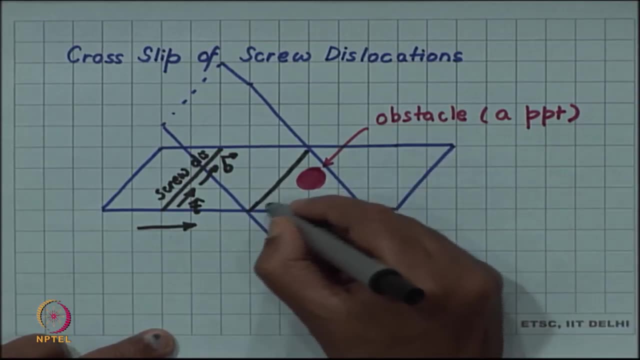 will be obstructed when it comes. let us say here: But if other plane is available for sliding, the dislocation can avoid this obstacle by a. if it is a screw dislocation, So then this other plane is also a slip plane. So if this 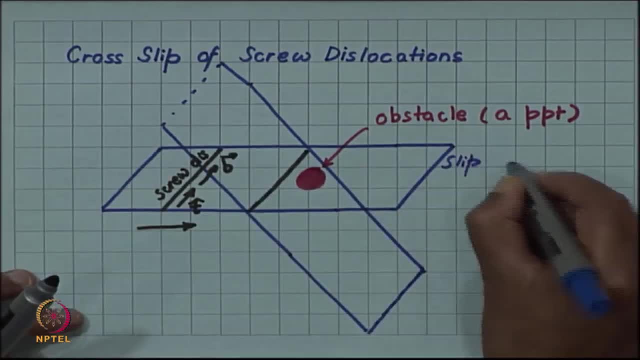 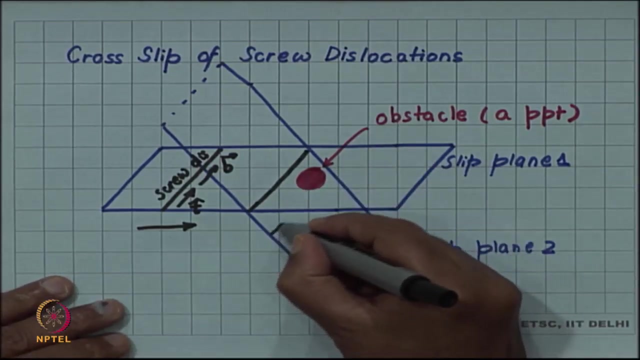 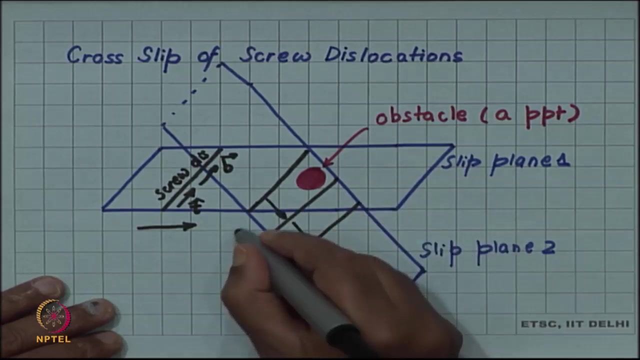 is a, this is a slip plane 1 and this is slip plane 2.. So the dislocation can avoid the precipitate particle by starting to glide in this direction. So this motion of the, of this change of the slip plane, is what we call cross slip. 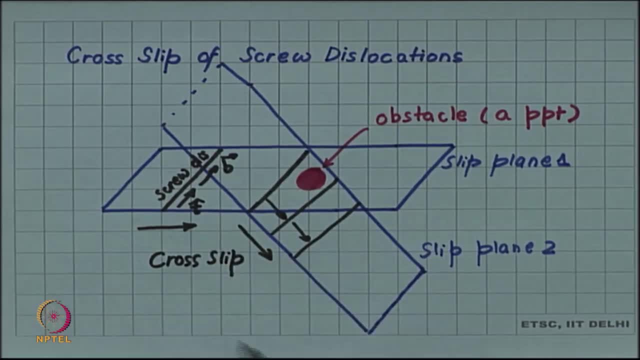 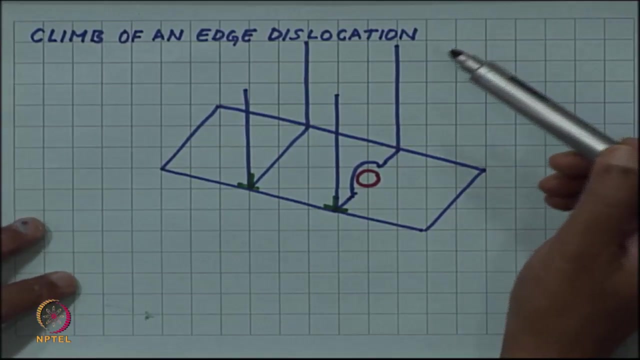 So if cross slip was not happening, the plastic deformation will stop at this point. but if cross slip is possible, then, since dislocation continues to move on a different plane, the plastic deformation will continue. __________________________. 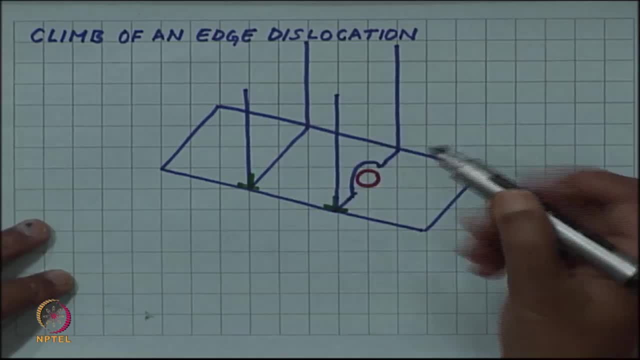 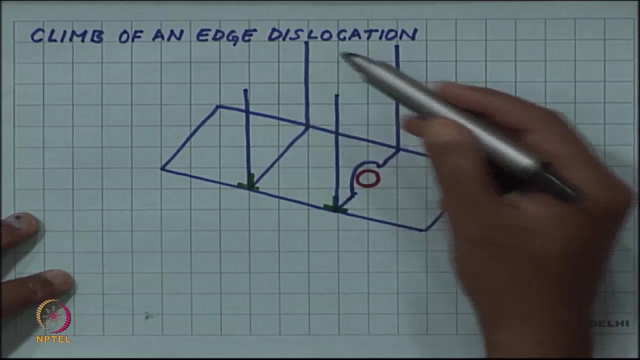 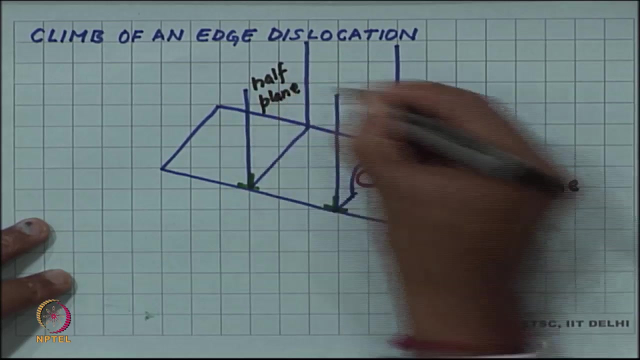 is climb of an edge dislocation. So we have seen, shown, a slip plane here. So let us call this the slip plane. So this horizontal plane here shown is a slip plane. The vertical planes which I have drawn here is the half plane of an edge dislocation. So this line, this 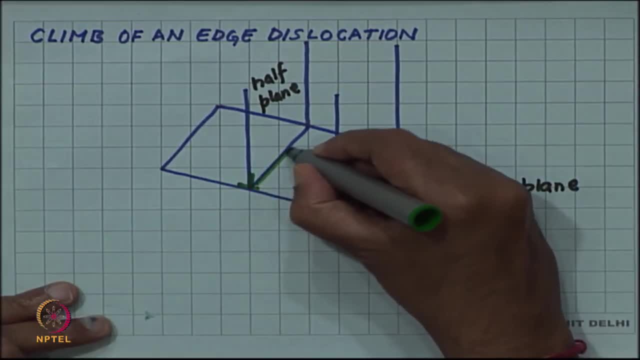 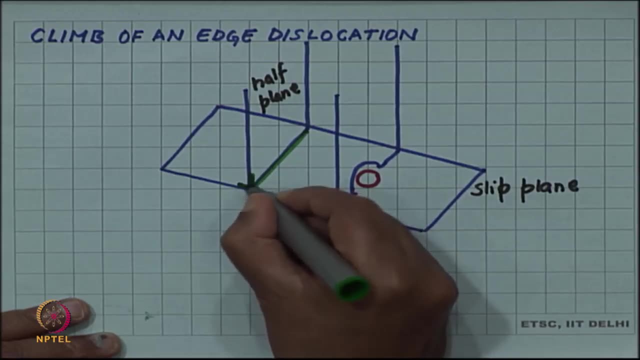 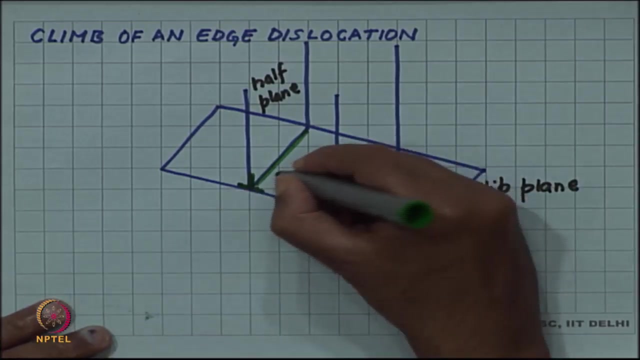 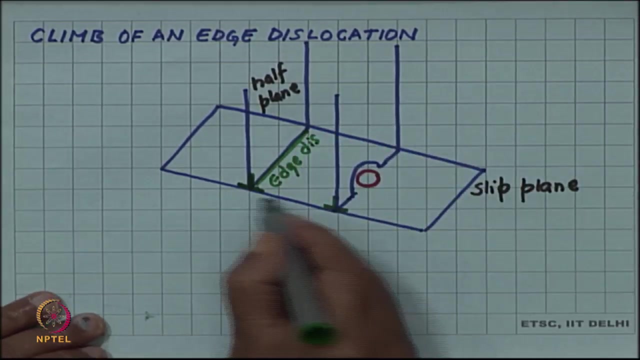 line will be the edge dislocation line and a, schematically, you know, we can represent it by an upside down t. So that is an edge dislocation, this is an edge dislocation and that edge dislocation, let us say, is moving in this direction And again there is a precipitate. 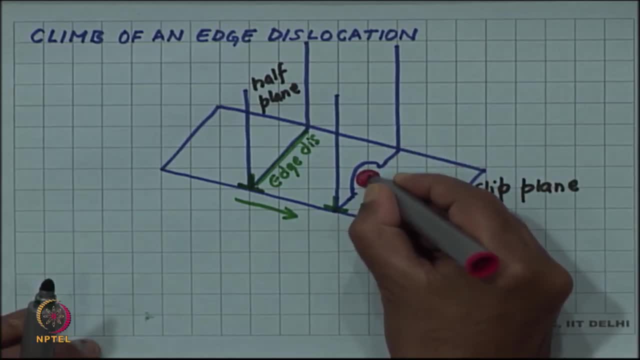 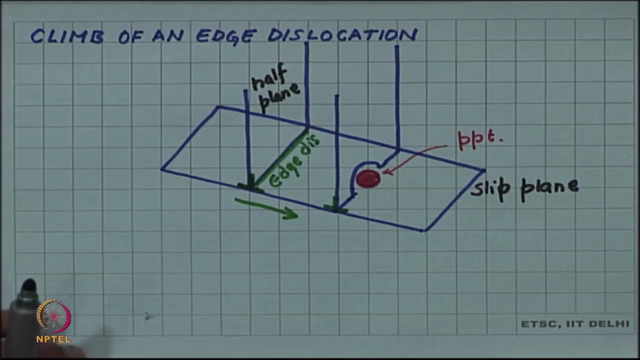 particle sitting on the slip plane is a precipitate particle which is sitting on the slip plane, Then in the normal situation the dislocation would be stuck by this precipitate particle and can move only at a continue to move only at a higher stress. We had considered that. 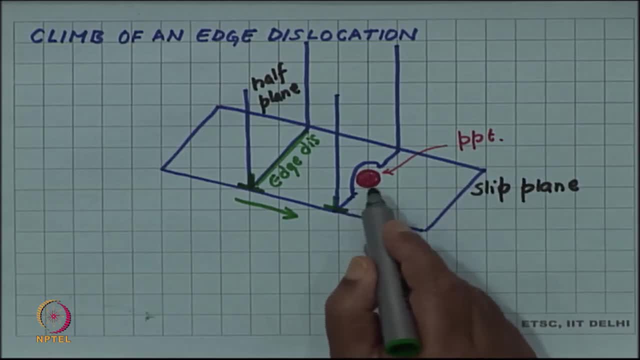 in precipitation hardening, Either the dislocation will have a higher stress than the precipitation hardening, So it is an edge dislocation to cut through the precipitate, which also requires higher stress, or it can form a loop around the precipitate, which again needs higher stress. 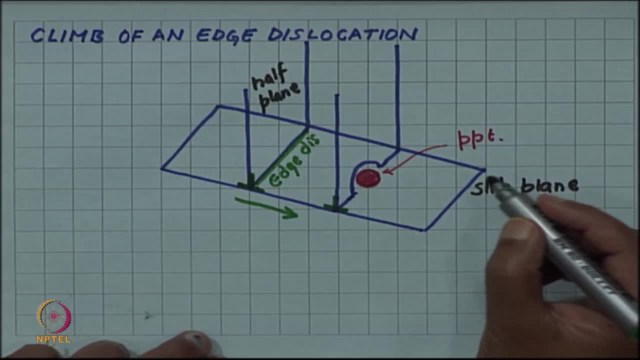 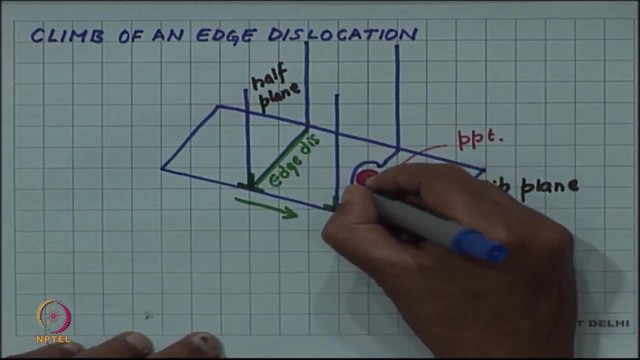 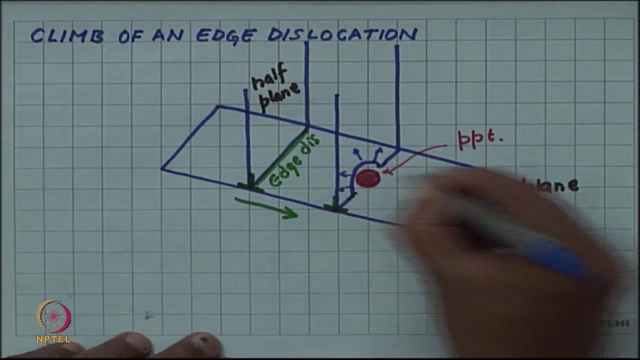 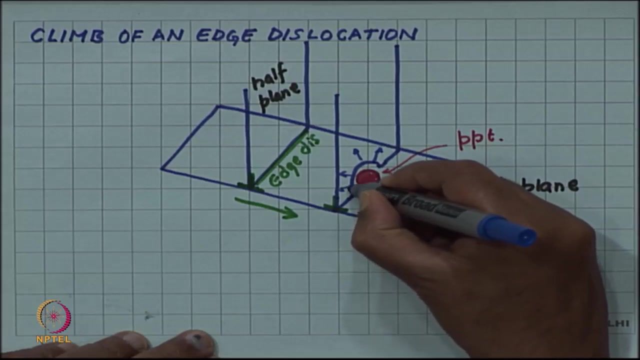 But if the temperature is high, like in case of creep deformation, then what can happen is that atoms at the bottom edge of the dislocation line can diffuse out, which is what we call climb up. So this segment of the dislocation line, this segment of the dislocation line has climbed. 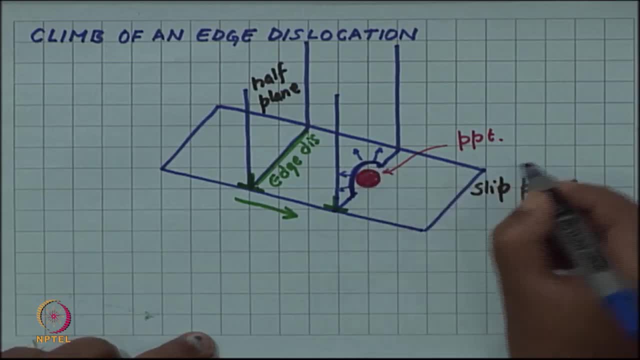 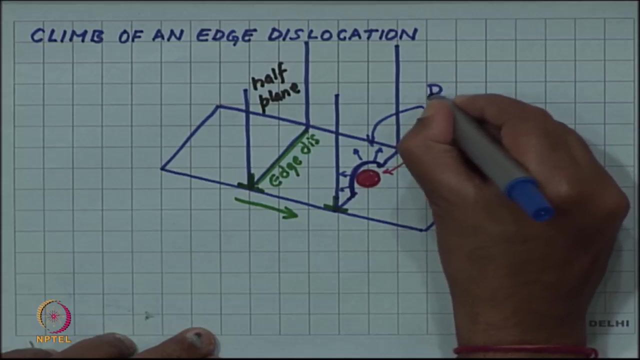 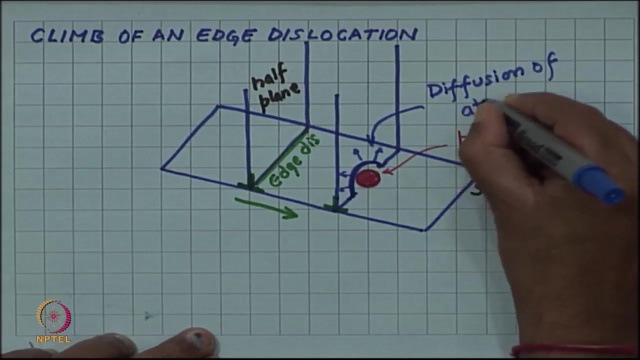 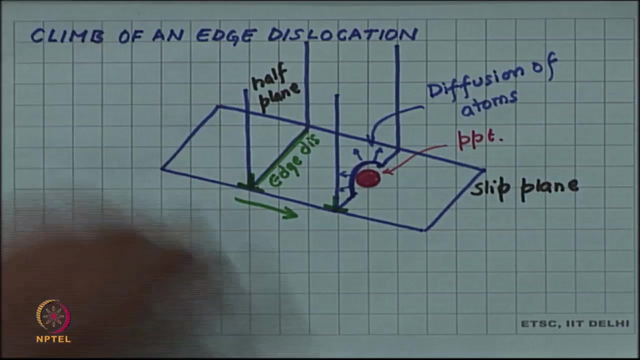 up and thus is able to avoid the precipitate, and the dislocation line can continue to move. This does not require any higher stress, Only requires a higher temperature for these diffusion to happen. So diffusion of atoms are involved in the climb of edge dislocation. 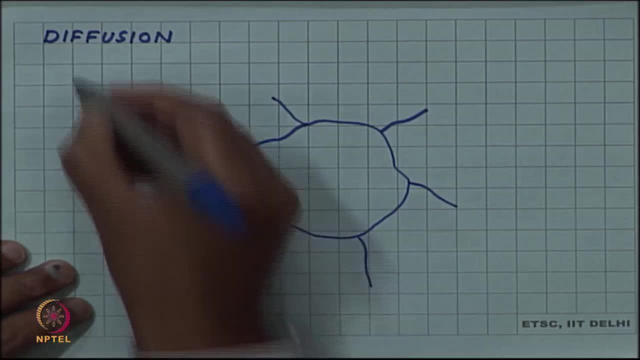 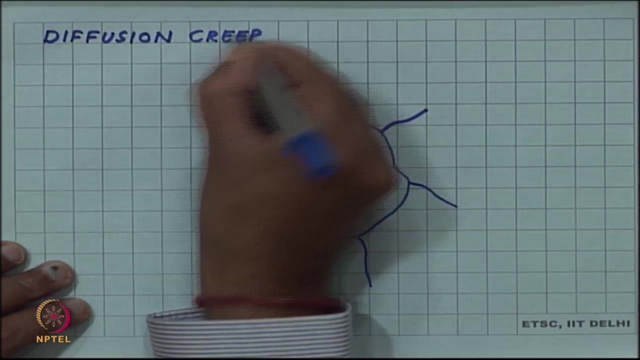 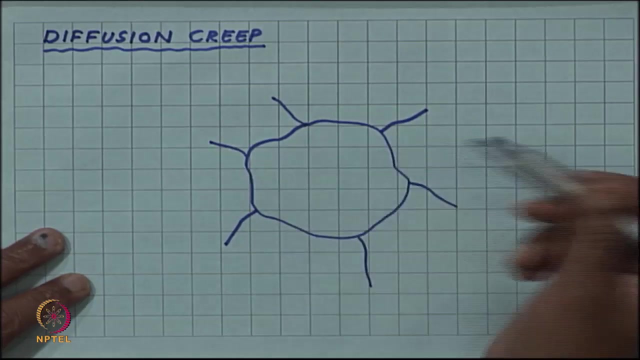 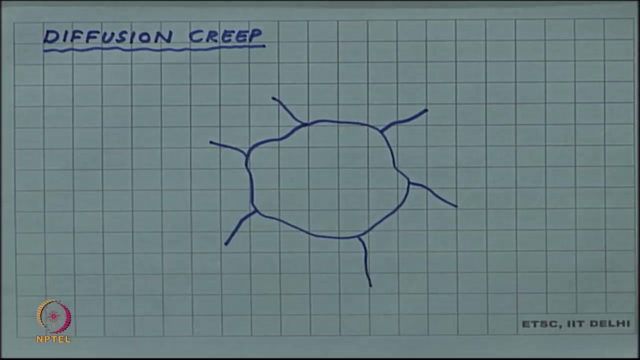 Now a dislocation free mechanism is So called diffusion, sometimes called diffusion creep or diffusion flow. So suppose this is showing a. this is an schematic of a grain and these are all a grain boundaries. and if this grain is subjected to a stress, if this grain is subjected to 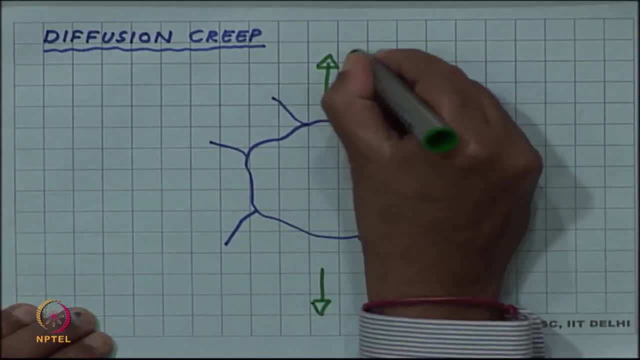 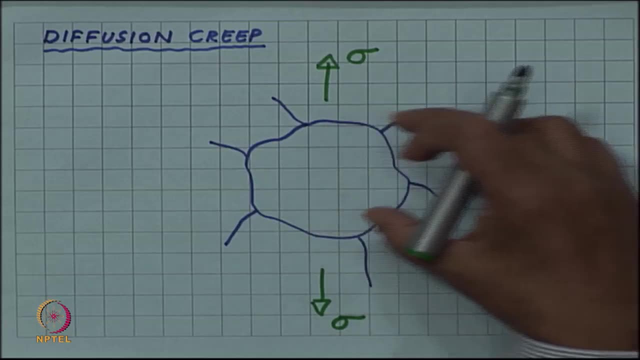 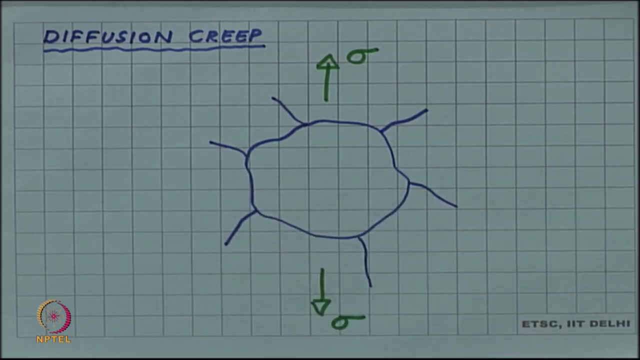 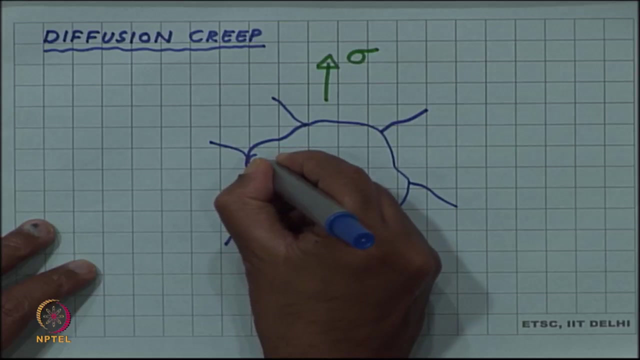 A uniaxial tensile stress, then you know that the grain will try to elongate in the direction of the stress, whereas will try to compress in the direction perpendicular to the stress. This elongation and compression, of course, can be obtained by dislocation motion, as it 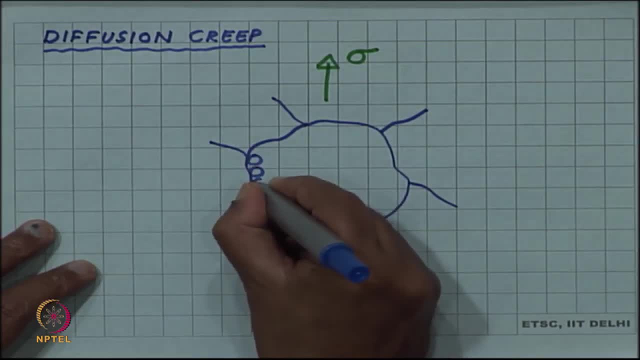 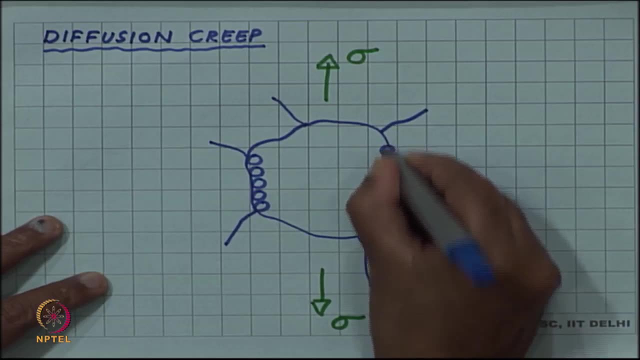 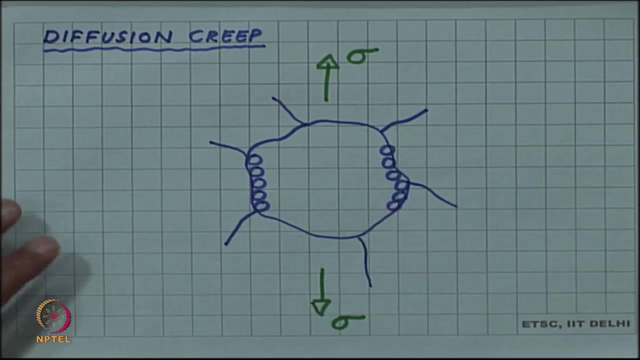 happens in low temperature But at higher temperature, since diffusivities are higher And atomic jumps are easier. One mechanism which is possible: that atoms which are on grain boundaries perpendicular to the stress axis- sorry, the grain boundaries parallel to the stress axis- They can move to grain boundaries perpendicular to the stress axis. 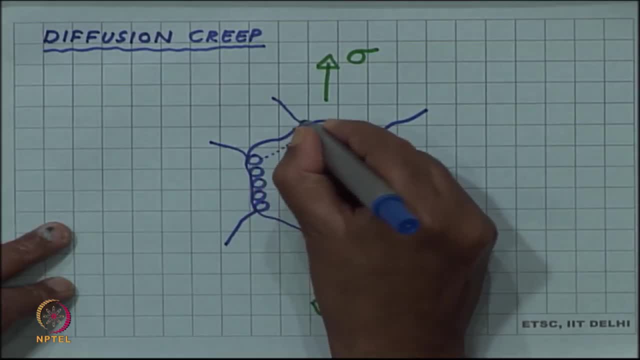 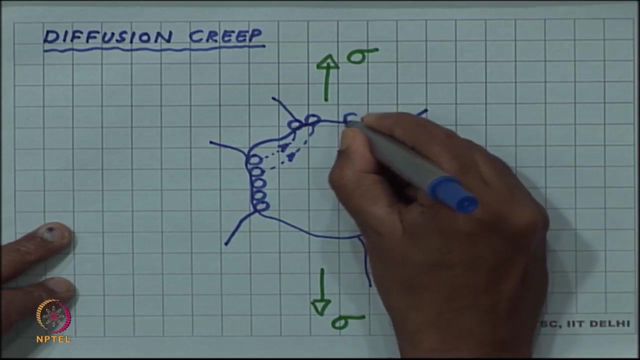 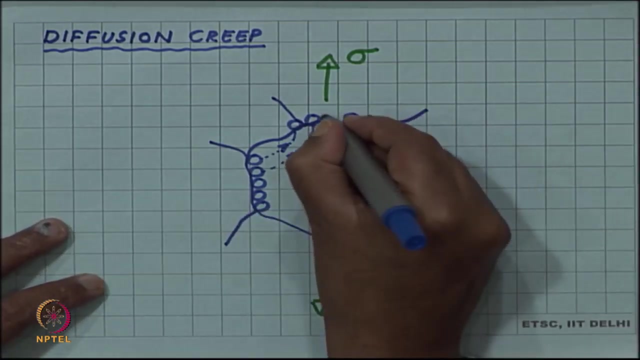 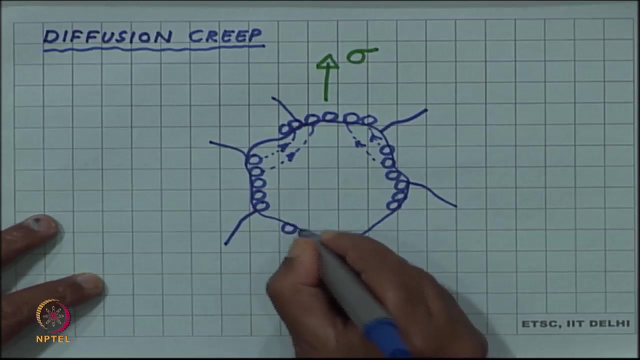 So if this atom moves from here And let us say This atom moves and joins here, this atom moves and joins here. similarly, this atom moves and joins here. So let us say, atoms migrate this way. So if these atoms migrate and join, then you can see. and similarly, on this boundary we 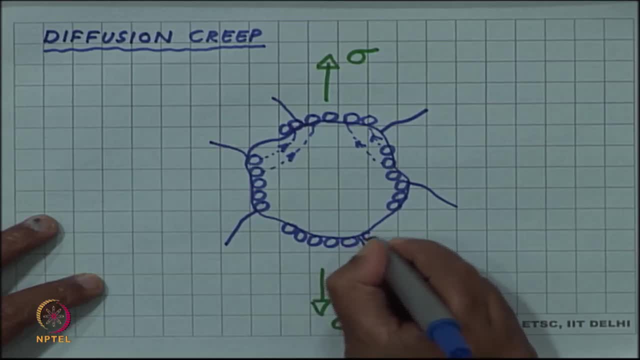 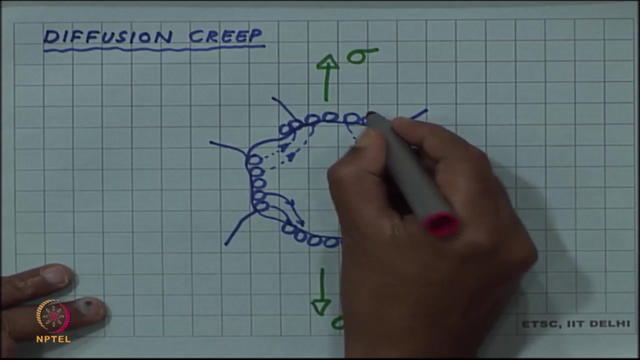 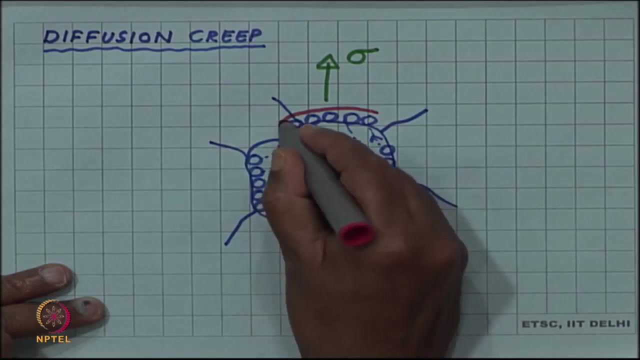 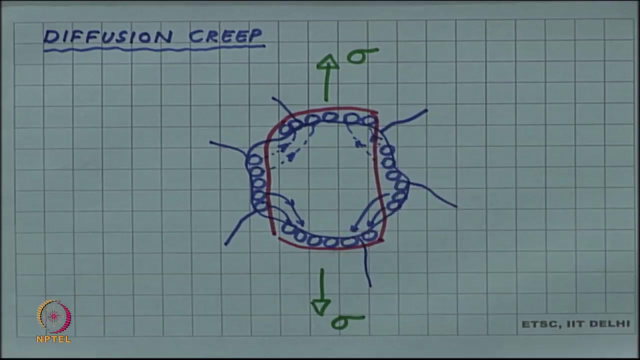 can have Atoms which have migrated from this side. So if this happens, then you can see that the size of the grain is increasing along these boundaries but is decreasing on this side. So after the diffusional migration, The grain shape will be something like this, which is exactly what this is. stress is trying. 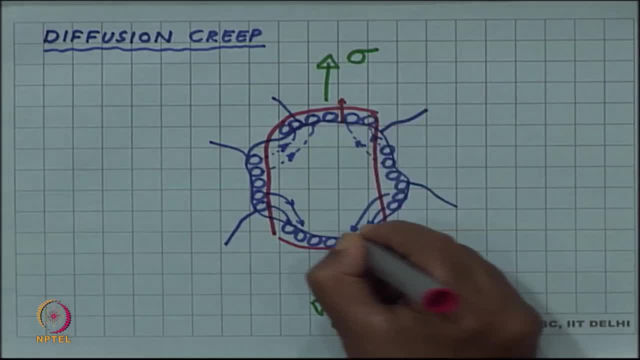 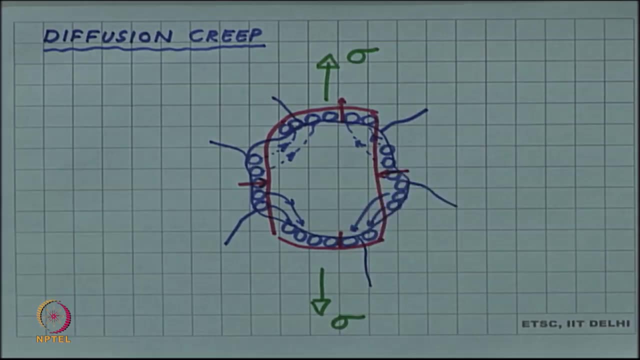 to do is to increase the length in this direction and contract the dimension in this direction. So you can see that this, in increment in length, as well as transverse contraction, can simply be achieved if the atoms migrate in this way. such migration is not possible at. 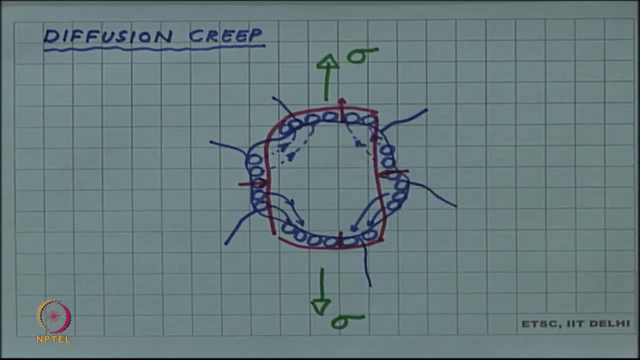 low temperature, But at higher temperature, due to higher atomic mobility and higher diffusion rate, such migrations are possible. this is, and this is a diffusion which is not governed by fixed law in the simpler form which we had talked about, that is, diffusion due to concentration gradient. because there is no concentration gradient here, only stress is applied. 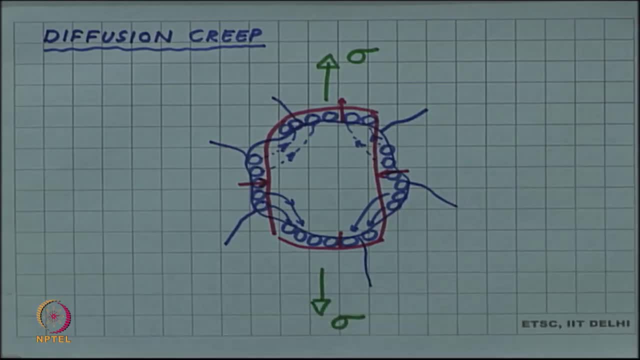 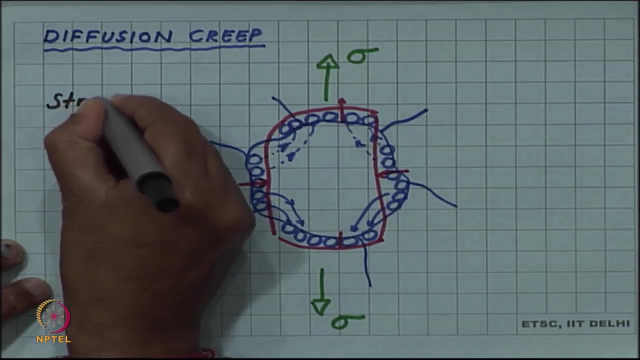 So this is a special kind of diffusion which we have not talked about earlier, but- and we are not going to discuss It in any detail here also- but we will simply note that this is a special diffusion mechanism, which is a stress assisted diffusion. 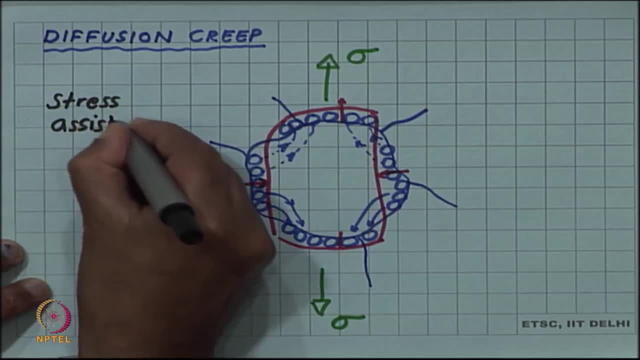 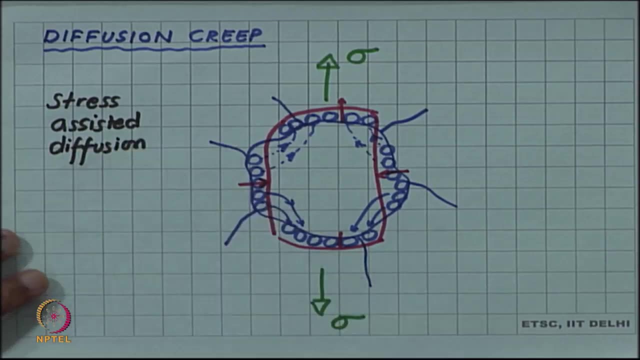 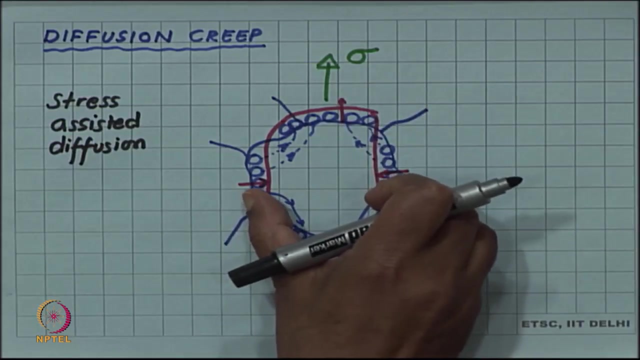 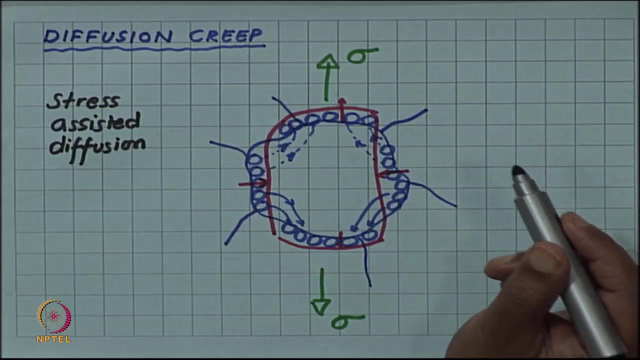 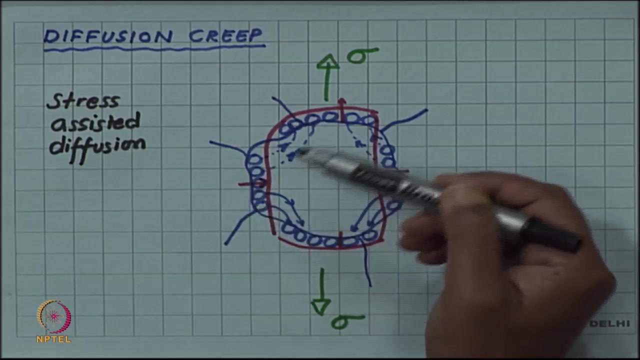 So these diffusion paths which I am showing is happening because the stress is trying to increase the grain size this way and decrease the grain size in this direction. So the atoms have a driving force for this kind of motion? obviously this is not. these atoms are atoms which make up the crystal. they are not interstitial atoms. 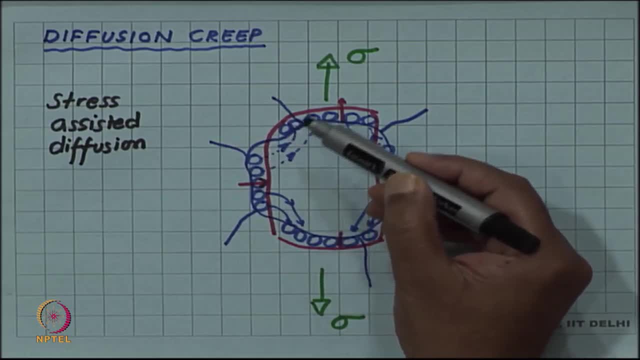 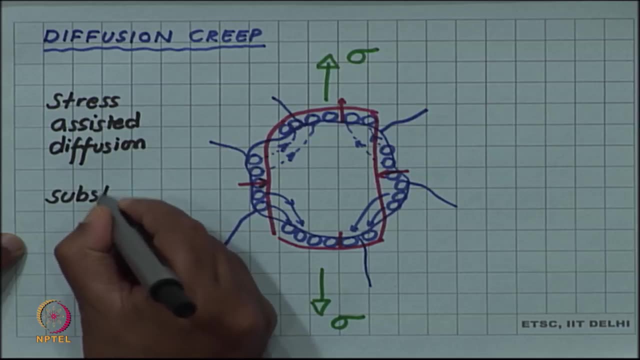 So these atoms can diffuse only by substitutional diffusion mechanism. So the diffusion is still substitutional. Ok, Thank you, Thank you, Thank you, sir. And for substitutional diffusion you need vacancy. this is vacancy assisted. and again, you know that vacancies are more available at higher temperature, at vacancy concentrations. 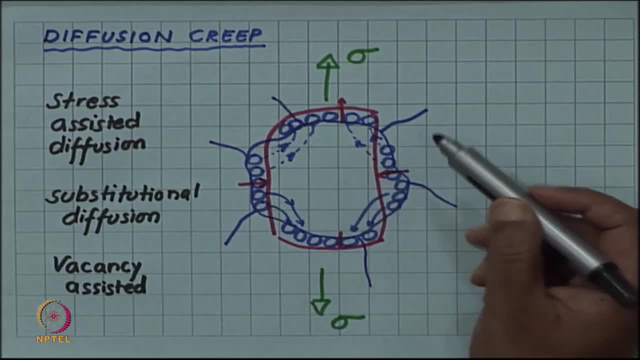 are higher at higher temperature. So this kind of diffusion is more possible because of higher temperature, which is most often used in the process Ok available during tree. So if we try to put the path of vacancy, if we do not look at, 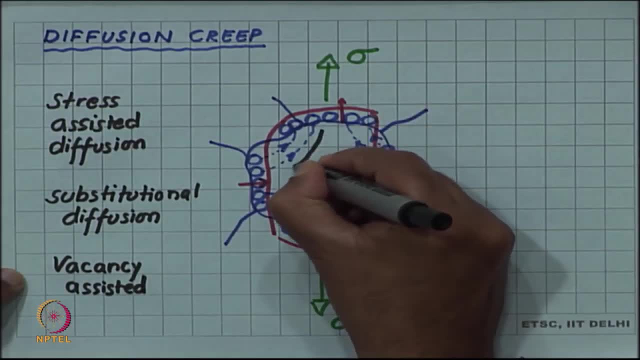 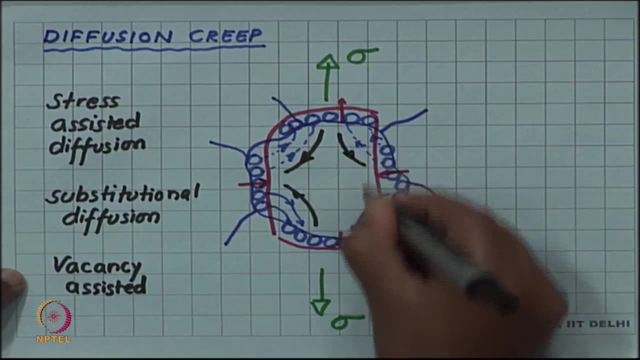 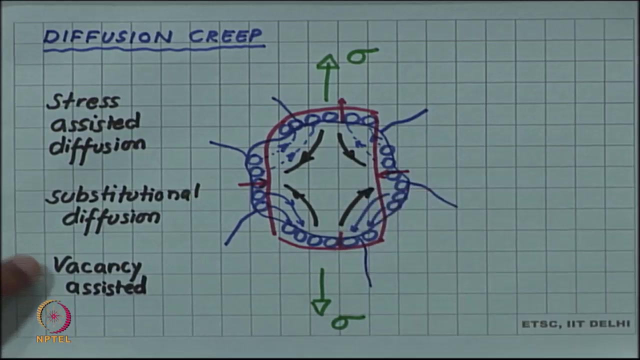 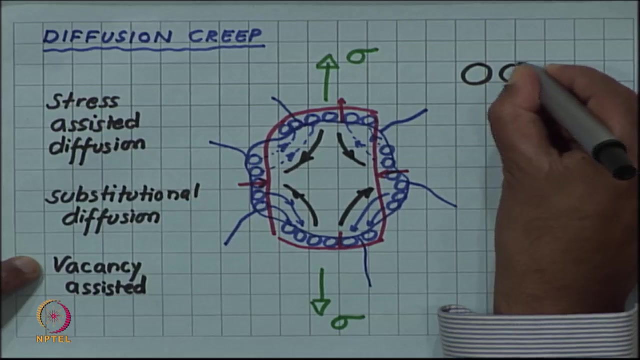 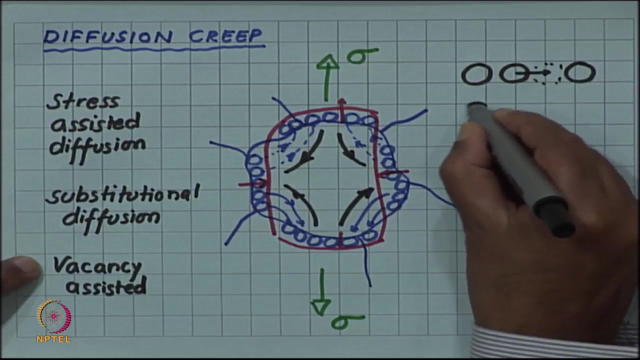 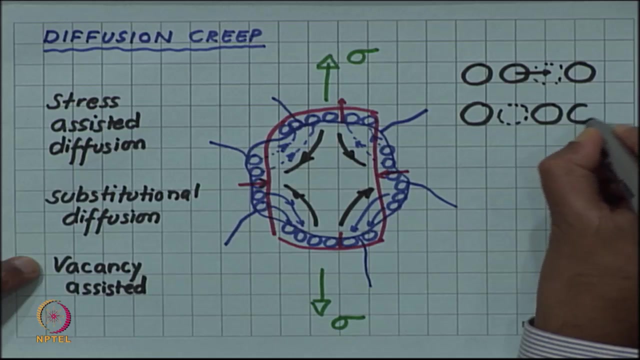 the atoms, but look at how the vacancy are migrating, So you can see that vacancy will migrate just the opposite way. This is, as you know, that if you have a vacancy and an atom jump, Atom jumps into a vacant site. So if I draw it like this, So this atom jumped into this vacant. 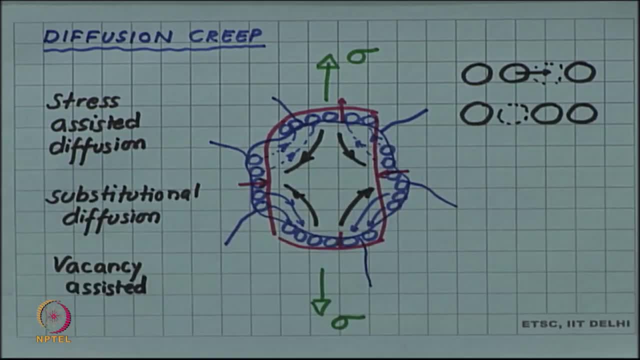 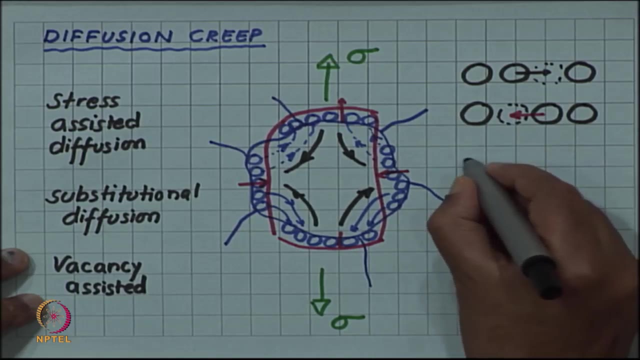 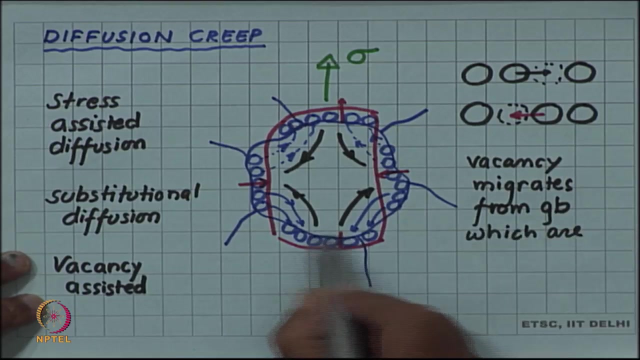 site. So, which means the vacancy which was there jumped in the opposite direction. So atomic migration direction in the vacancy directions are different and this is stress assisted diffusion- leads to vacancy migrating from grades, from grain boundaries which are- you can see the grain boundary, which are perpendicular. 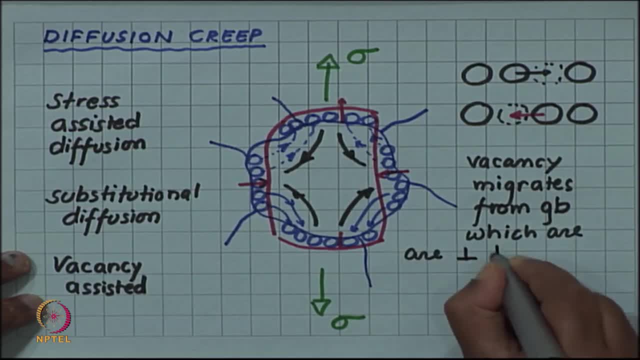 to stress y, two grain boundaries which are parallel to stress axis. So this is a stress assisted diffusion of vacancy which leads to diffusion creep. There is no dislocation required. but if vacancies move this way, the atoms move the opposite way and the deformation will. 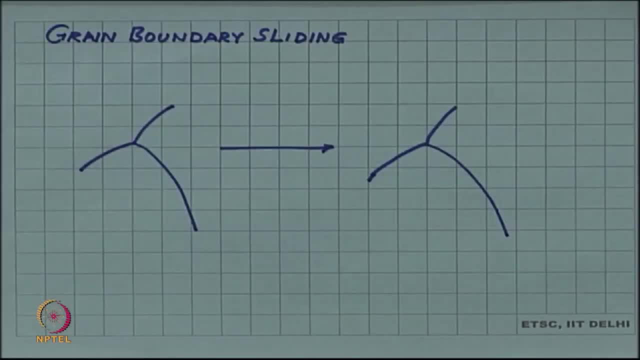 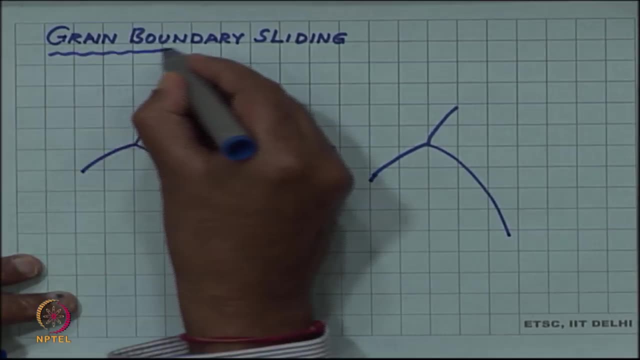 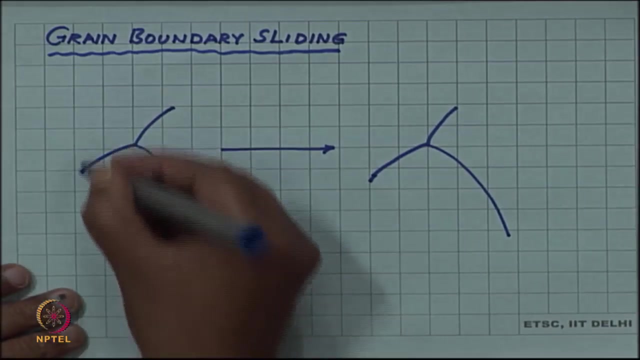 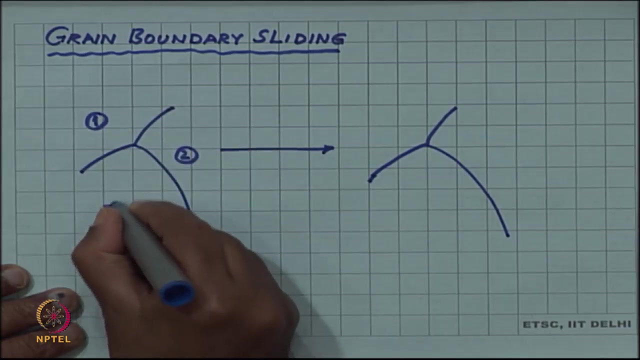 happen. Yet another diffusion mechanism, yet another deformation mechanism which does not involve dislocation, is the grain boundary sliding. This again happens at higher temperature. Here I am showing you a schematic of, let us say, three grains. This is grain 1, grain 2 and grain 3, grain. 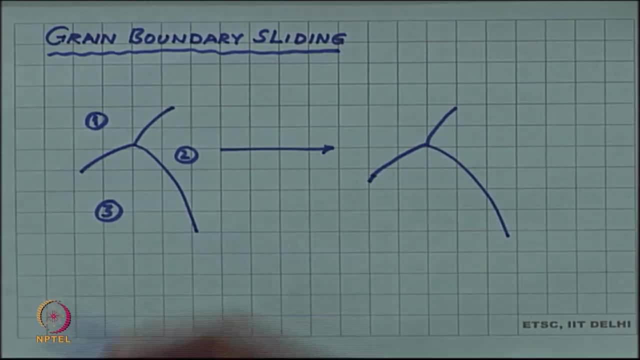 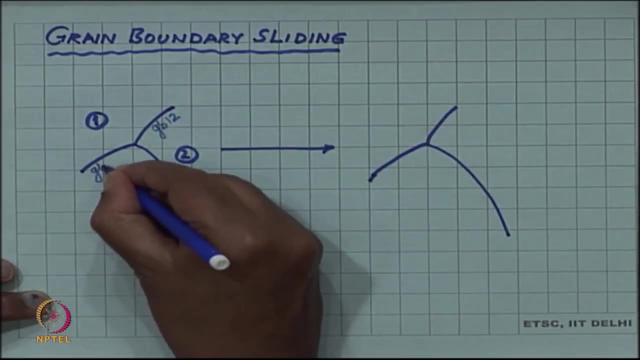 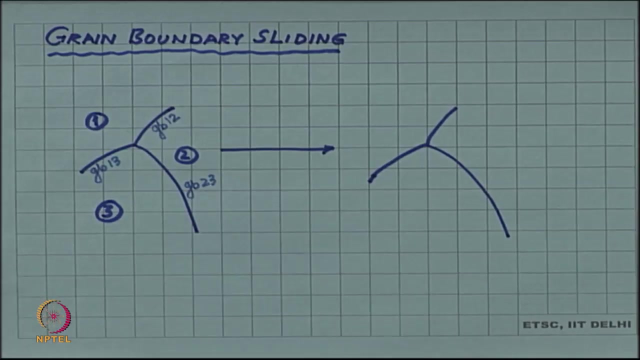 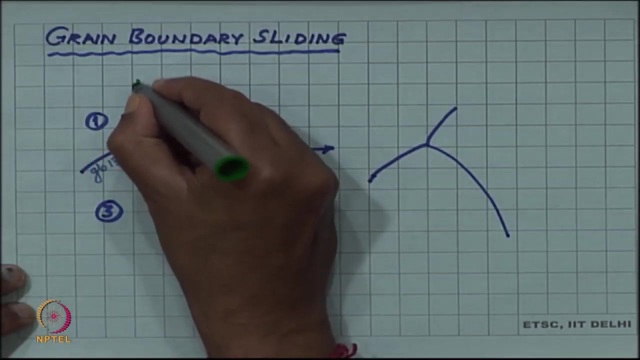 3, and these are the grain boundaries. So this is grain boundary 1, 2, grain boundary 1, 3 and grain boundary 2, 3.. And now, if this system is again subjected to stress, then at higher temperature. 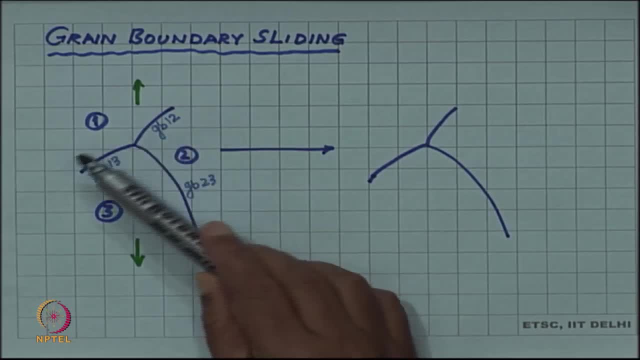 grain boundaries become weaker than the grains, So they act like somewhat a viscous liquid along the grain boundary. Liquid is a little stronger term, but they it is easier for the grain to slide on these grain boundaries at higher temperature, under the influence of. 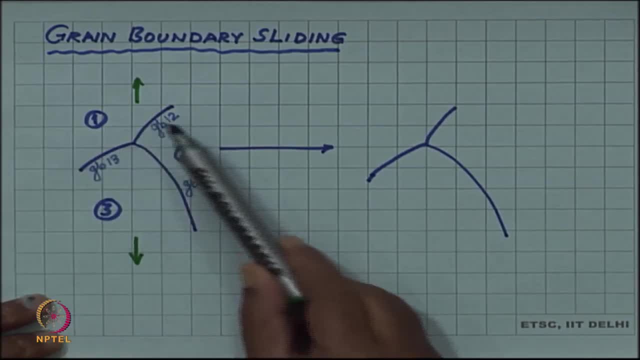 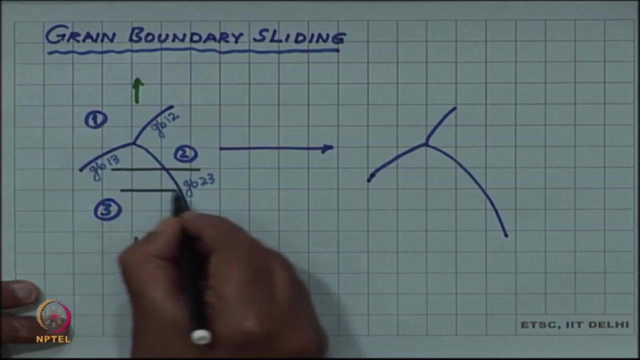 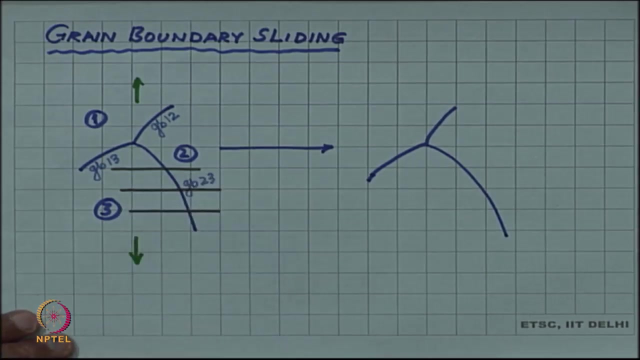 stress. So if shear stress is there on these boundaries, the grains can slide. This has been actually observed in experiments by drawing some test lines across the boundary. So suppose if I draw test line across this boundary before deformation, which are continuous across the 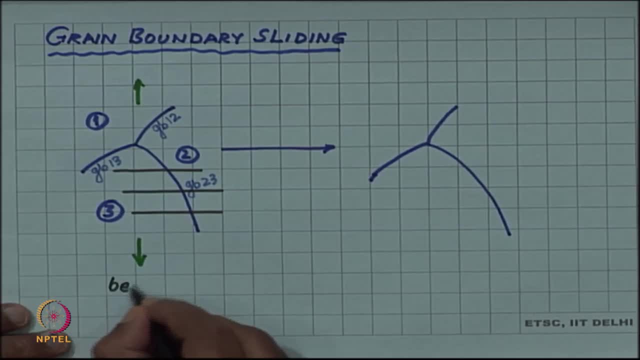 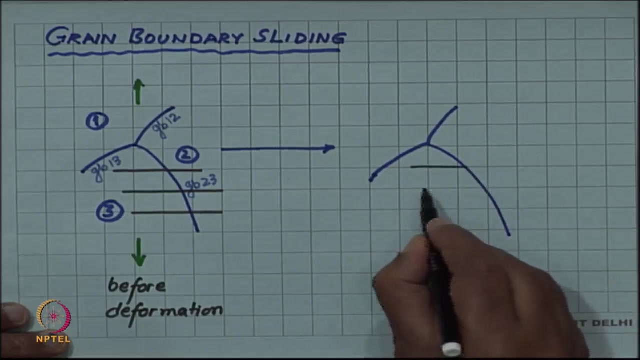 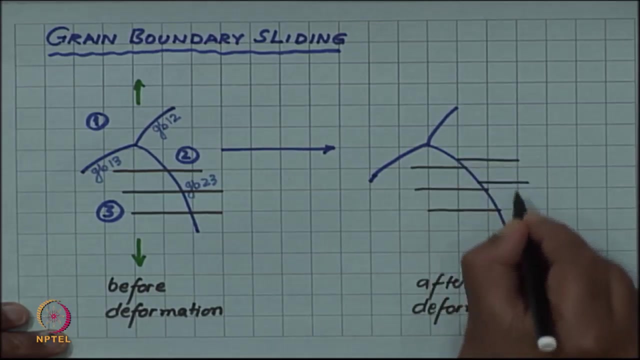 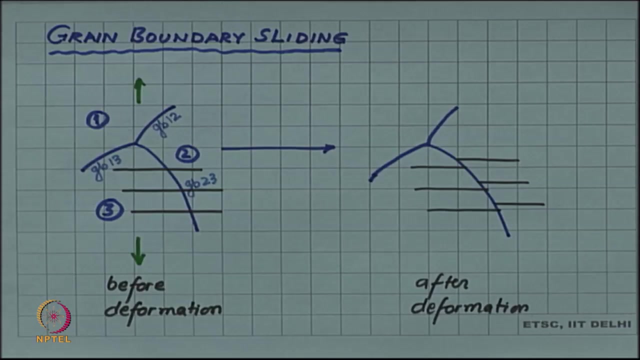 grain, then after deformation. So if I draw a test line across this boundary before deformation, then after deformation one finds that these lines have become discontinuous. The continuity across the boundary is lost and you find something like this: So which means this grain? 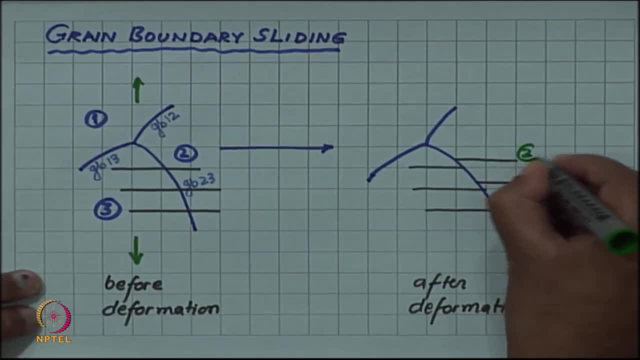 grain 2. It has slid over the boundary at higher temperature. So this is what I have said in the exposed area and this is what you will find in the boring landscape. So you went back from the lavoro and you found these different lines in the boundary. There is no. find out the core. 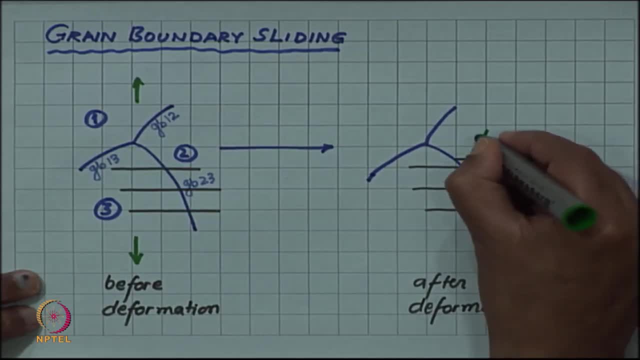 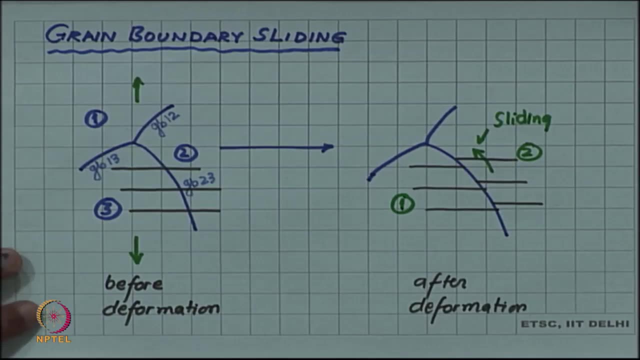 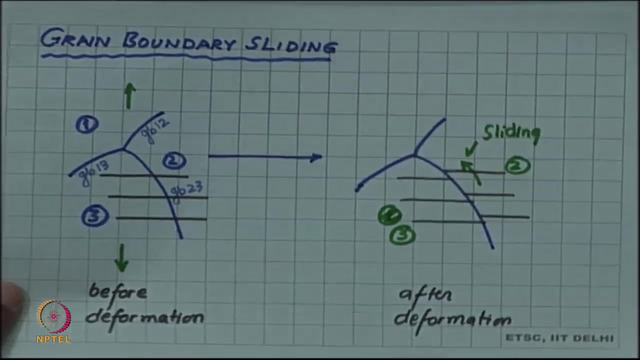 upwards with respect to grain 1 across the grain boundary. So grain 2 and grain 3 are sliding on the grain boundary to 3.. So this is yet another mechanism which is possible, and this is again possible at high temperature, because at high temperature only. 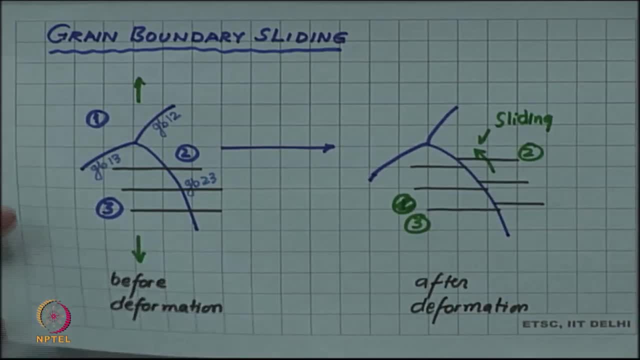 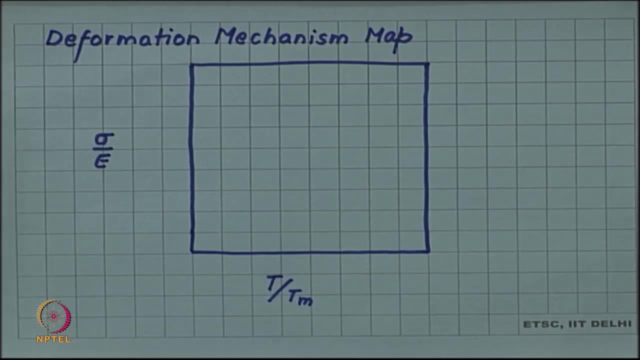 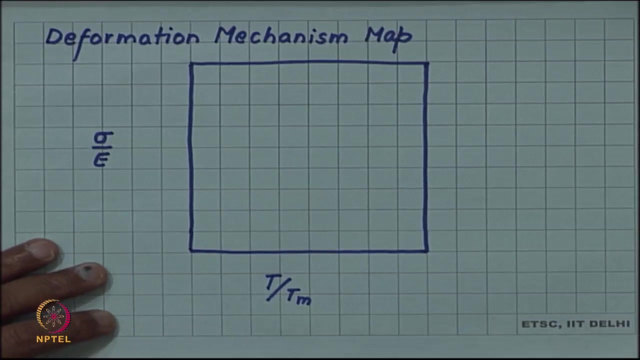 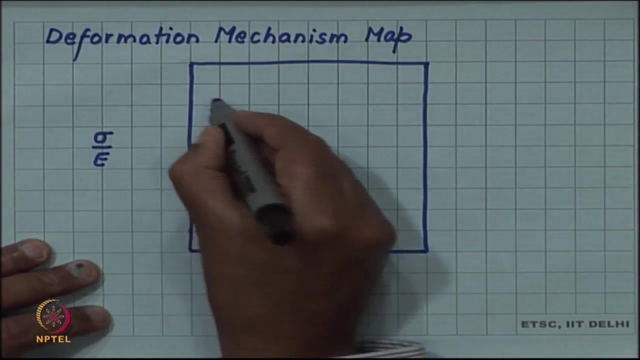 the grains become weaker, the grain boundaries become weaker and allow for this kind of sliding. Finally, an interesting way to present the deformation as a function of a stress and temperature is what is called the deformation mechanism map, and a simpler form of this map is what we will draw now, So we have something called yield stress. 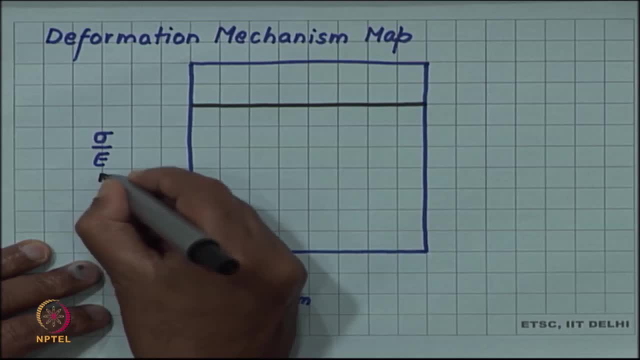 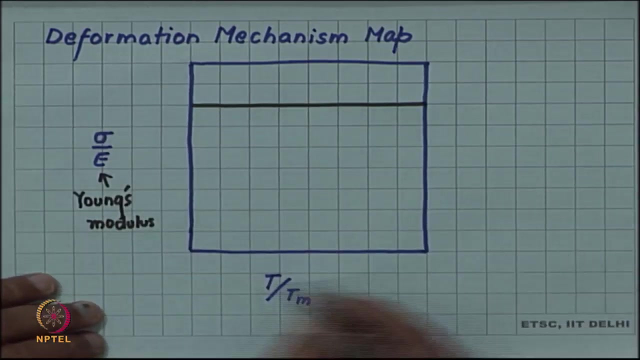 So the y axis is stress versus the modulus Young's modulus. So y stress is the y axis is stress, but it is normalized with respect to Young's modulus. and x axis is temperature, but it is normalized with respect to the melting point.